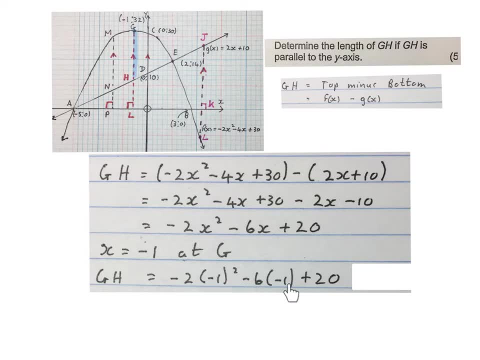 Substitute it into this expression that I just worked out. Everywhere, in the place of x, I put a minus 1.. And I simplify this expression now. Then you write g. h equals 24 units. Stop the video and get your brain around this. Next they can ask me to work out the length of. 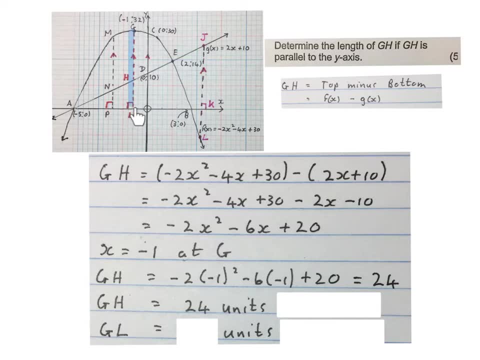 g, l, There is g and there is l, that total length, And the answer will be 32 units. They gave us the coordinate of g, which was minus 1 for x and 32 for y. That means it's 32 units from the top to there. 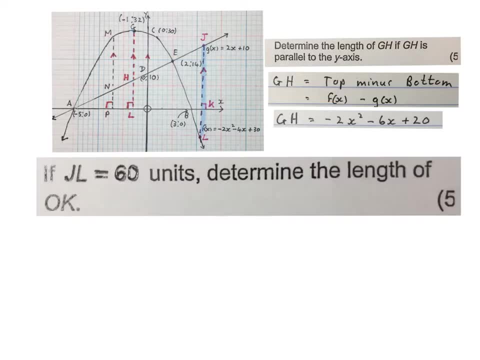 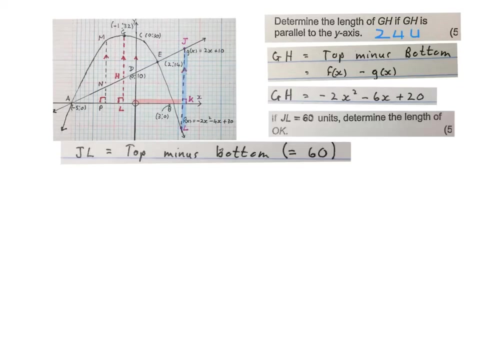 No calculations necessary. The next question reads: if j, l is 60 units, determine the length of o, k. They say: if this blue line is equal to 60 units, how long is that red line from the origin to k? Firstly, we have to find an expression for the length of the blue line. 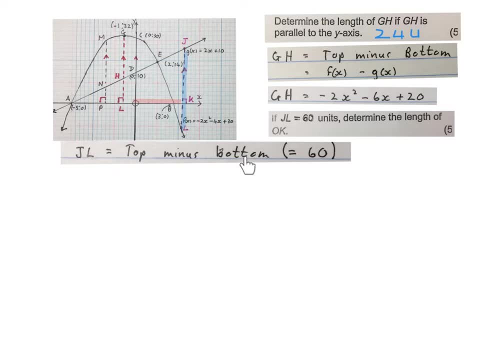 So we write: j l equals top minus bottom and j? l is 60. At the top we now have the straight line. So we have g of x minus f of x. We fill in the expressions in brackets, simplify them, and here we have an expression for j l. 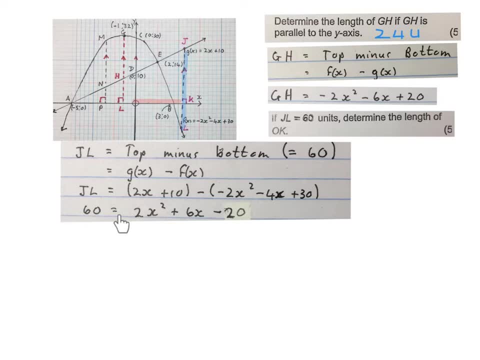 But we know that j? l is 60, so we go: 60 equals this expression. Of course, it is now a quadratic equation: i minus 60 on both sides and I get 0 equals to 2x squared plus 6x minus 80.. 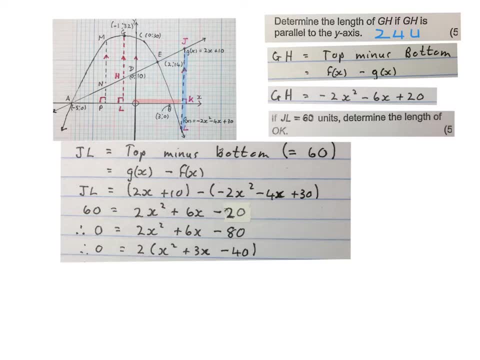 Now we can solve for x: Factorize a common factor out Factorize and get two values for x: x equals to minus 8, or x equals to 5.. Now we look at the line again and we see it's here on the positive side of the x axis. so it can't be x equals to minus 8, it's not on this side. 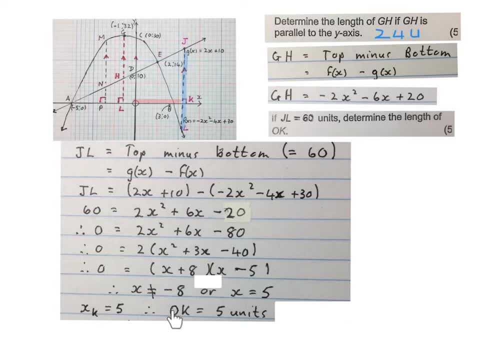 Like I said, x at k will be 5, so the length of o k, that red line, will be 5 units. Please stop the video and get your brain around this. The next question says m? n is equal to 20 units. how long is o p? 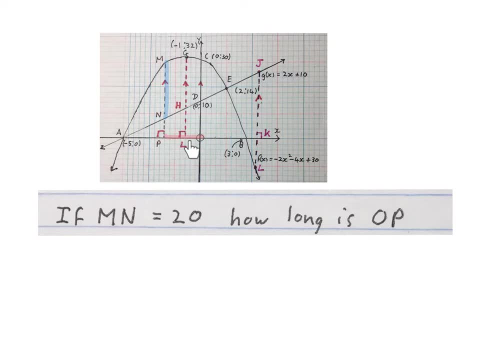 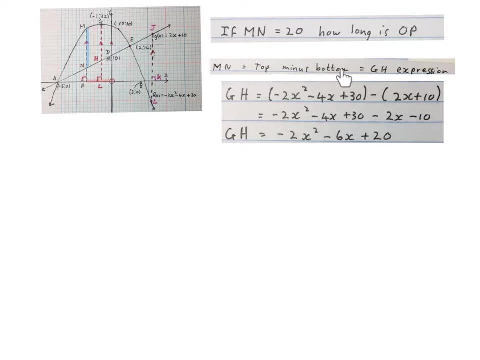 So that blue line is 20 units. how long is that red line? Now to get an expression for the length of m n, it's also going to be top minus bottom, but that's the same as what we did for g, h. 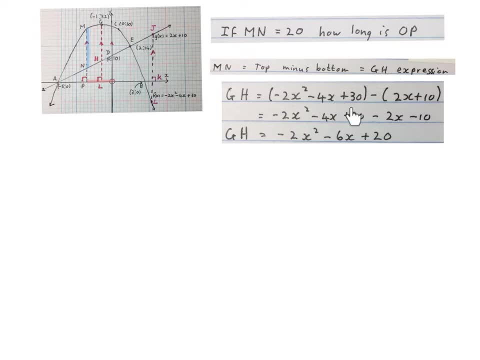 We took the top, which is the parabola minus the straight line, and got the answer: minus 2x squared minus 6x plus 20.. Both m n and g h will use this. Both m n and g h will use this. 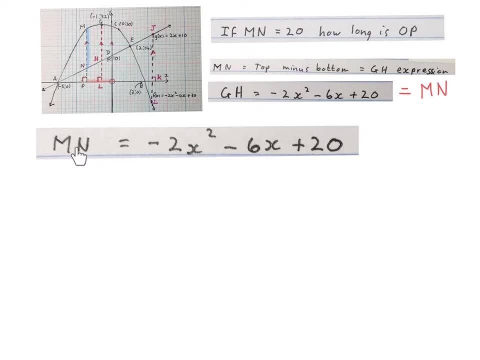 Now we can start. we can say m, n equals to this expression, equals to 20 units, And we'll have an equation looking like this: a quadratic equation Minus 20 on both sides to get a zero on that side. 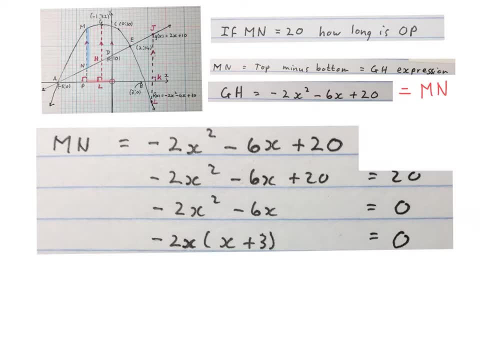 Now we solve for x. Now we get 2 answers: x equals 0 or x equals minus 3.. So x is not allowed to be 0 because it's not over there on the y axis. x is not allowed to be 0 because it's not over there on the y axis. 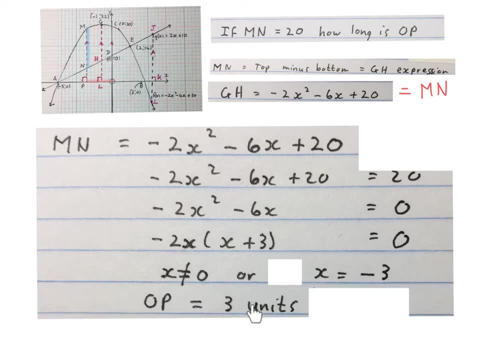 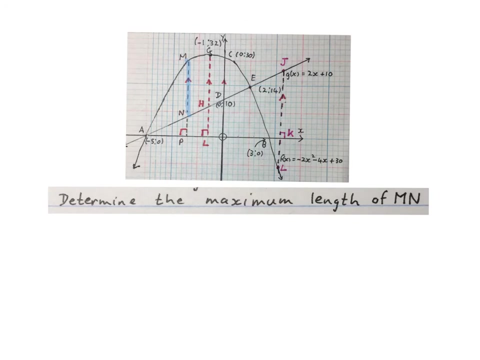 to the left. so OP will be three units long. If you can't write minus three, although the X value over here is minus three, the length is three units. Please stop the video and get your brain around this. The last question on these two graphs is: determine the maximum length of MN? We have a quadratic expression for: 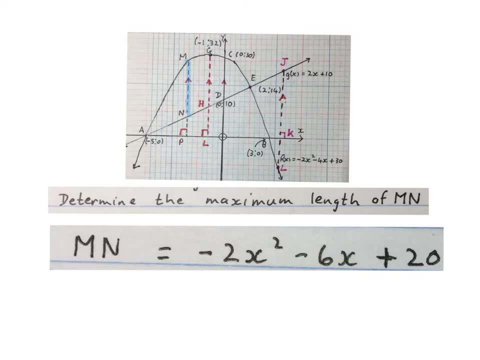 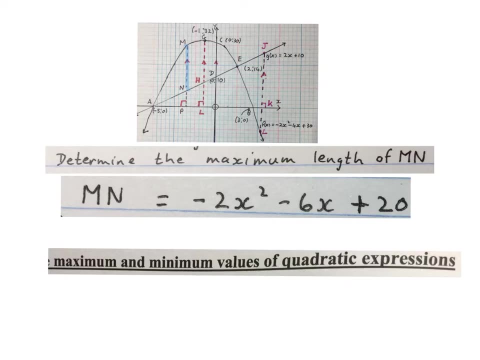 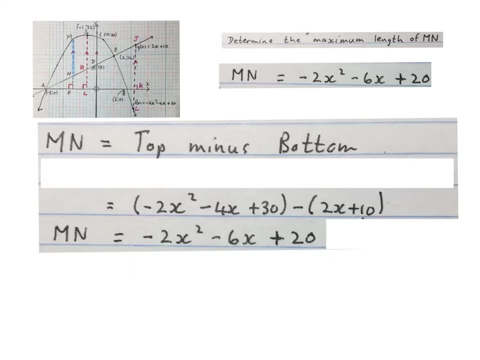 the length of MN, which we got from top minus bottom, and I advise you to go and look at the video that says maximum and minimum values of quadratic expressions. There we gave you more than one way to find this answer. Let's quickly take this question from the top. So, firstly, you find MN's expression with top minus. 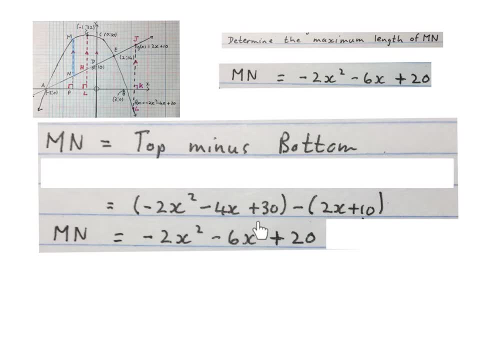 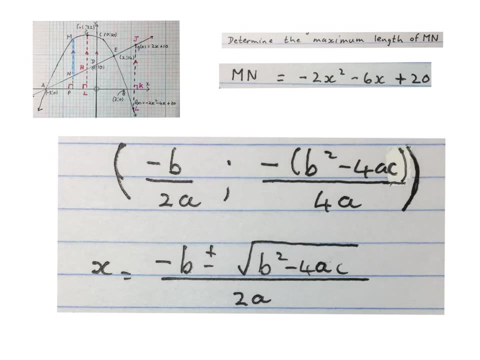 bottom You take the parabola minus the straight line and get this new expression which I wrote down here. Then I advise you to use this set of formulas- We use it in quite a few places in maths- to work out that we use this formula to find out. 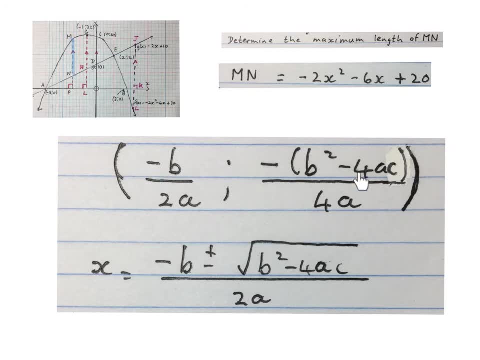 what the answer is Where this blue line will be a maximum. Use this formula to find the maximum value of this blue line using this expression. Just quickly want to mention it. This is not so difficult to remember. this formula, There it is in your quadratic. 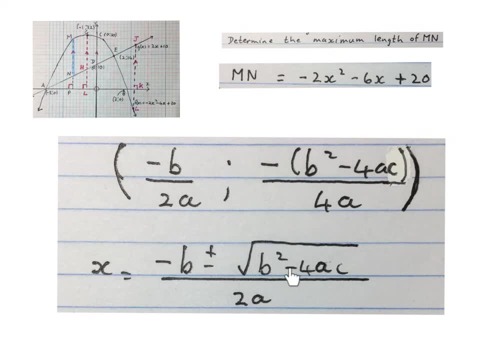 formula and that B square minus 4 AC. you already know from your quadratic formula. Just make that 2 of 4 and put the minus in front there. So not so difficult to remember this formula. This is where it is a minimum or maximum, and 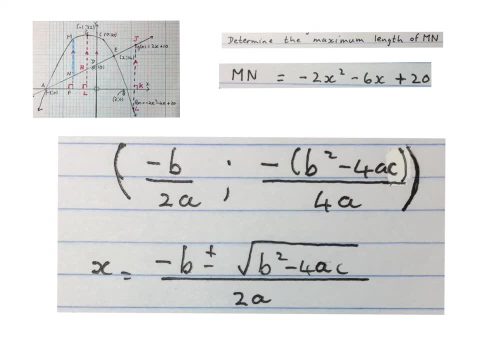 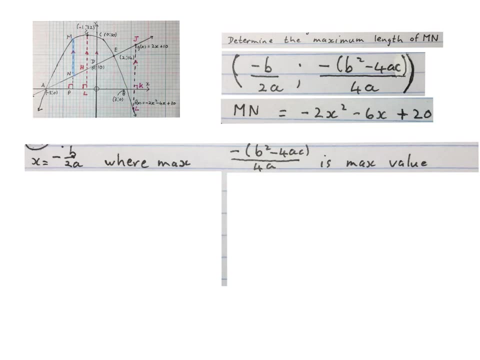 this is what the minimum, or maximum is in maths. Don't get lost in my words now. So, like I said, this formula will give us the maximum value. they asked us. Determine the maximum length of MN From our expression. we know that A is minus 2- there it is. B is minus 6- there it is. and C is 20. 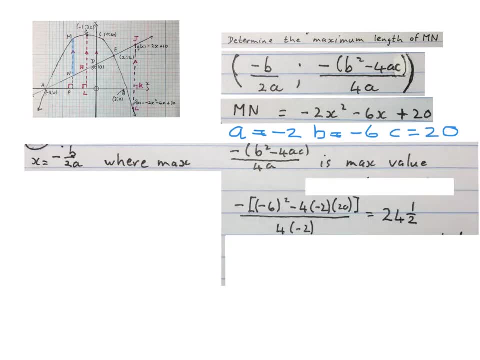 at the back here. Substitute it into the formula and get the answer 24 and a half. You just write the sentence. the maximum length of MN is 24 and a half Units. If they asked you where will it be a maximum, We will use this formula. Plug. 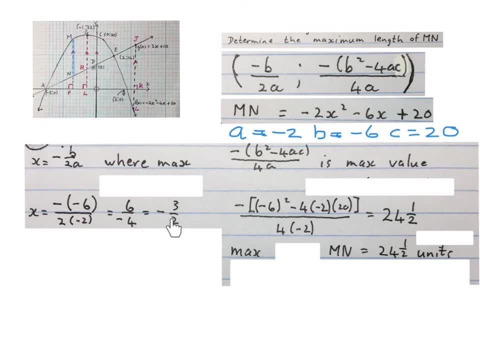 in the values of A and B and get your answer. This was not part of the question, but you could then say: the maximum length of MN is 24 and a half units, where X is minus 1 and a half. So X is minus 1 and a half on this side. This MN will be. 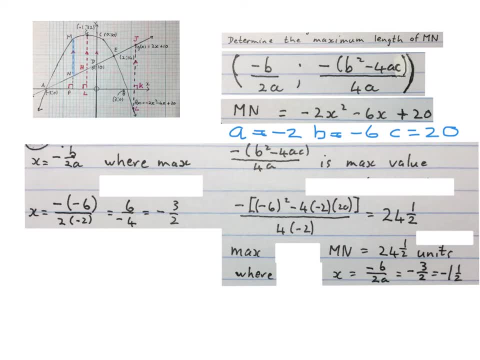 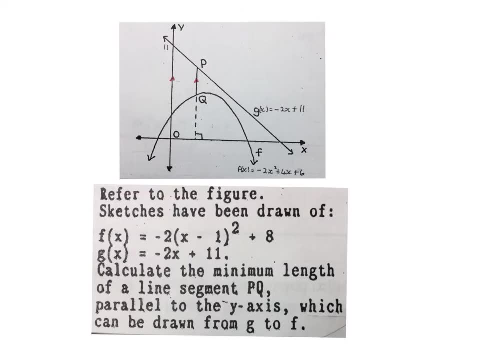 the longest it can get. Remember the question was only determine the maximum length of MN. Please stop the video and get your brain around this. Here is the last question. They gave us this sketch with a parabola and its equation and a straight line and its equation. The question reads: refer to the figure Sketches have. 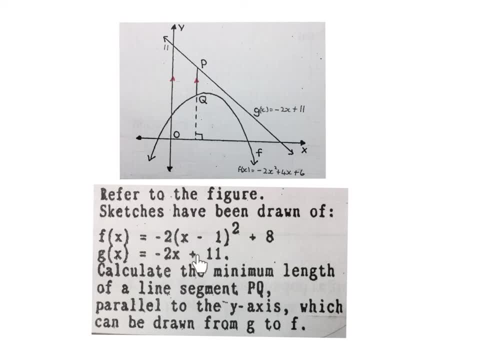 been drawn of F of X, that's the parabola, and G of X, the straight line. Calculate the minimum length of a line, segment PQ. that line there, Parallel to the Y axis, which can be drawn from G to F. So they want the minimum length. 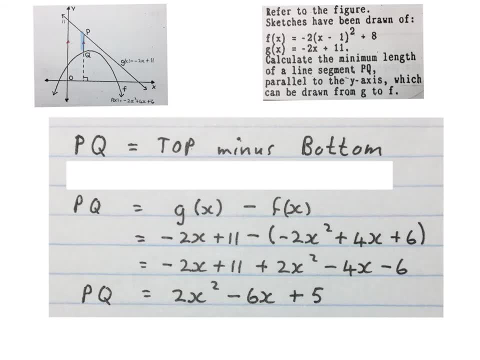 of the line PQ. I'm not going to spend a lot of time on this. To find PQ's expression I go top minus bottom. So PQ is G of X minus F of X, This one minus this one, Filled it in, simplified it and